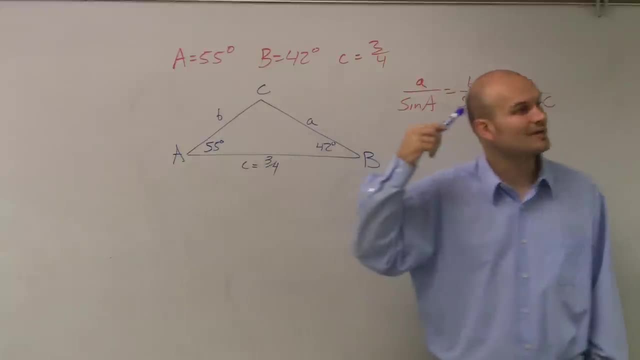 a little intuitive sense and look at it and say, well, I am given two angles of my triangle so I can figure out what the side length of C is, or, I'm sorry, the angle of C, right? So I think a little bit to think about: oh well, I can figure out what the side of C is. So all I do 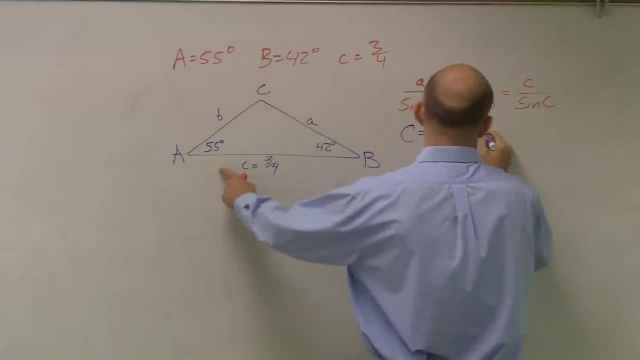 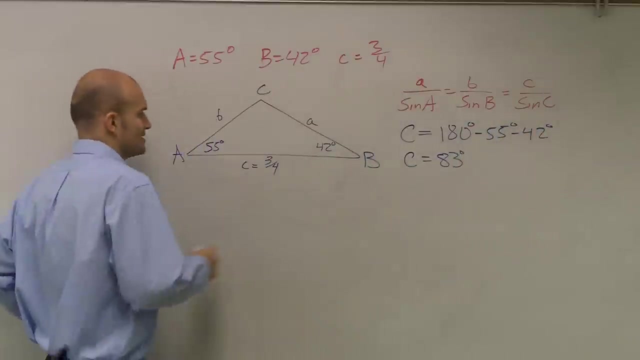 is sine of our angle, C is equal to 180 degrees minus 55 minus 42. And so those two added up together give me 97. So therefore, C is going to equal 83 degrees. right, Put all the degrees in there. So C equals 83 degrees. So I can figure out what the side length of C is. So I can figure out. 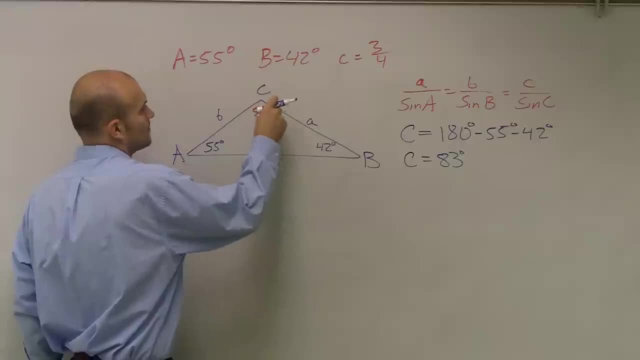 what the side length of C is. So I can figure out what the side length of C is. So now I can apply the law of science. So I'm actually going to do it twice. So, since I have these two, and I have both, 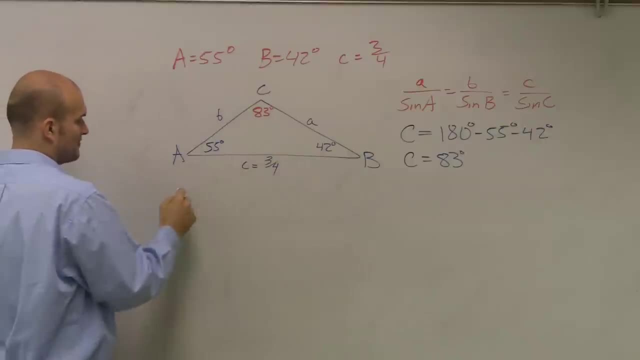 of these angles. I'm just going to set it up. I'll say set of 3 fourths. I'm just going to convert it to a decimal. all right, It's pretty easy to convert 3 fourths to a decimal, So I'll just use. 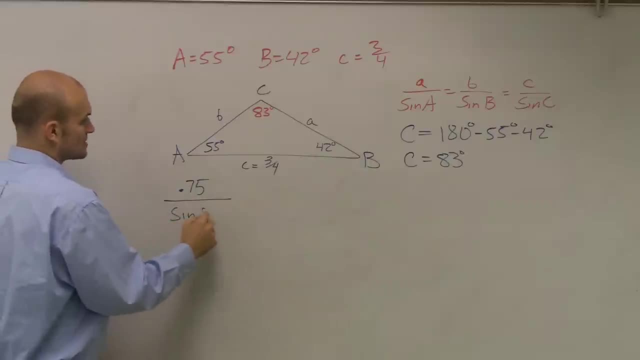 it as a decimal, because I'm going to be primarily using my calculator. Sine of 83 equals A over sine of 55. And let's do that again. 0.75 over sine of 83 equals B over sine of 42. So I'm going. 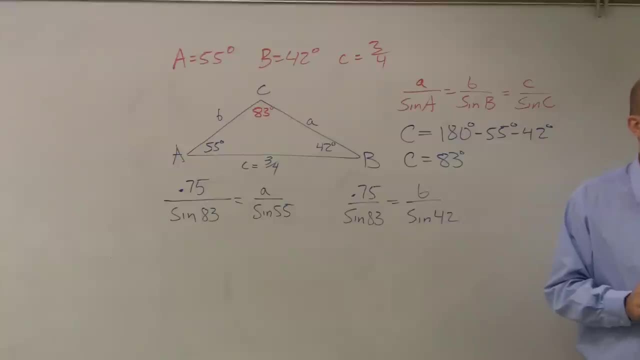 to do both these problems, one for finding A, one for finding B. So the next thing to remember is cross multiply. So when I cross multiply and then isolate my variable, I'll have- I'm going to just kind of skip a couple steps right, Because I've kind of shown this before- 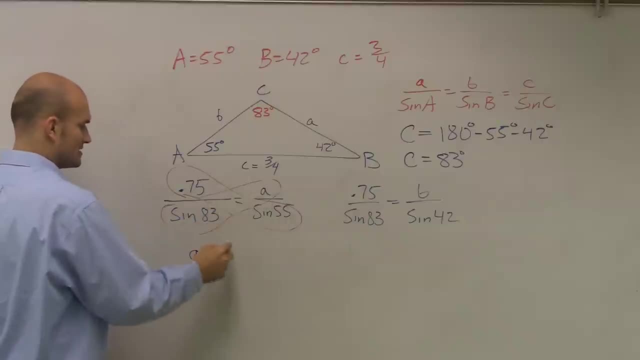 Is that? okay? So cross, multiply, I'll get A equals. these two multiplied by each other, So 0.75 times sine of 55. And then when I have to isolate this variable A, I'm going to have to divide by sine of 83.. Okay, So A equals And then this one. when I solve for B, I'll have 0.75.